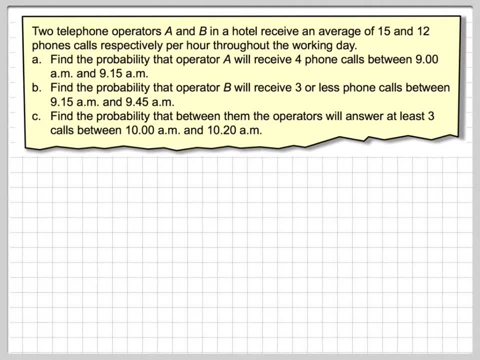 Right in this video we're going to look at two telephone operators with a changing time interval and see what effect that has on the possible probability calculations. Okay, so we've got two telephone operators, A and B, in a hotel receive an average of 15 and 12 calls. 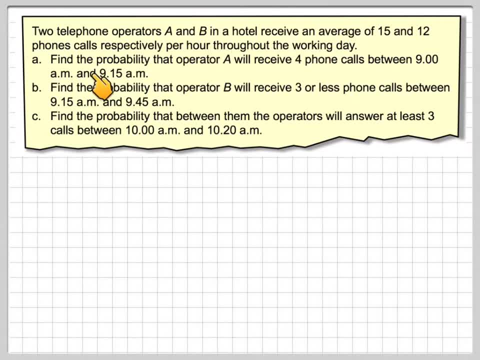 respectively per hour throughout the working day. Find the probability that operator A will receive four phone calls between 9 am and 9: 15 and then find the probability that operator B will receive three or less phone calls between 9: 15 and 9: 45 am, and find the probability that between them the 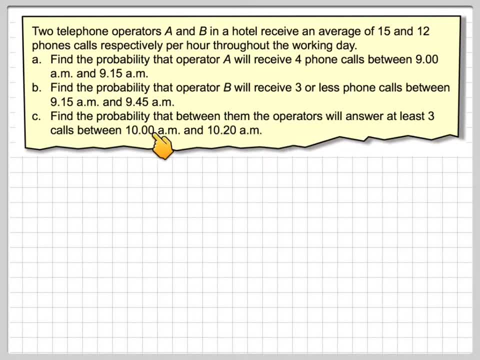 operators will answer at least three calls between 10 am and 10: 20 am. So the time interval in the first part is 15 minutes, the time interval in the second part is 30 minutes and the time interval in the part c is 20 minutes. Okay, and we've got averages per hour, so per 60 minutes. 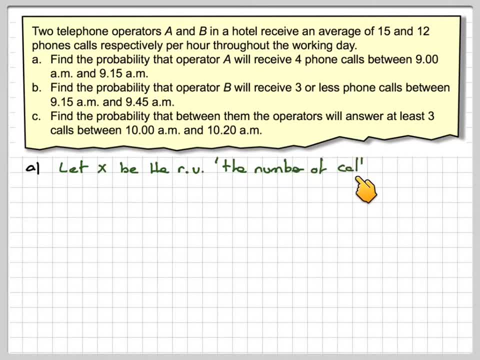 So let x be the random variable, the number of calls answered per 15 minutes by operator A. We know that in 60 minutes operator A receives 15 calls and therefore in 15 minutes he receives 15 divided by 4 calls, because the time period has been. 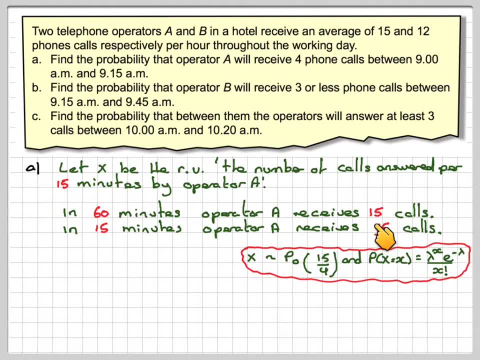 reduced. So 60 divided by 4 gives you 15. so we have to do the same here. so x will be plus on 15 over 4, and a probability that x is equal to x is lambda to the power of x, e to the minus, lambda over x. 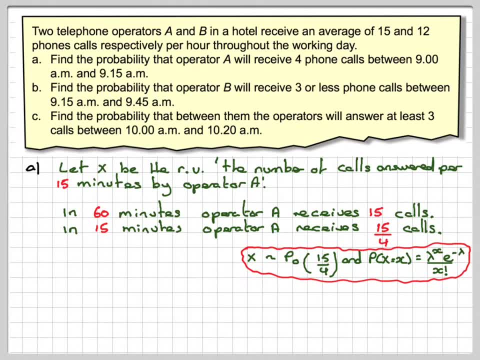 factorial. We want to receive exactly four phone calls, as probability x is equal to four. so we're going to just kind of calculate this one. so it's going to be 15 over 4 to the power of 4, e to the minus 15 over 4 over 4, factorial. You could change that to a decimal. 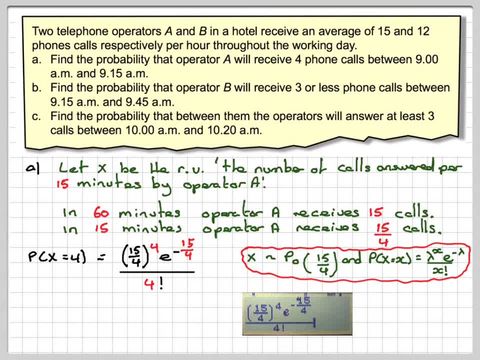 if you prefer to, but it is possible to work with these new calculators in fraction mode. There it is and there is the answer. So we get 0.19378025, which gives me 0.19423- significant figures. Okay, part b find the probability that the 37rd number for series 2.1.. 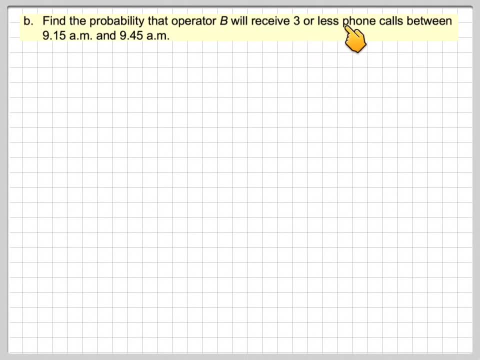 件事情, operations against the problem. find the probability that operators' positions balance at 0.19378025, which gives me 0.19423. significant figures. Okay, part b. find the probability that operators' Operator B will receive three or less phone calls between 9.15 and 9.45.. 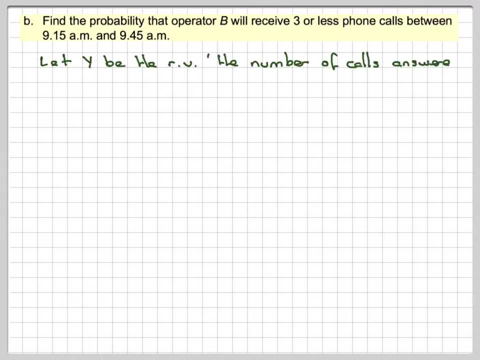 So let Y be the random variable, the number of calls answered per 30 minutes by Operator B. In 60 minutes, the question said Operator B received 12 calls. Therefore in 30 minutes it's going to receive half of that 12 divided by 2, which is 6 calls. 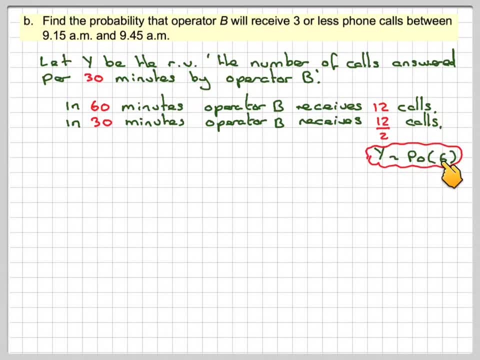 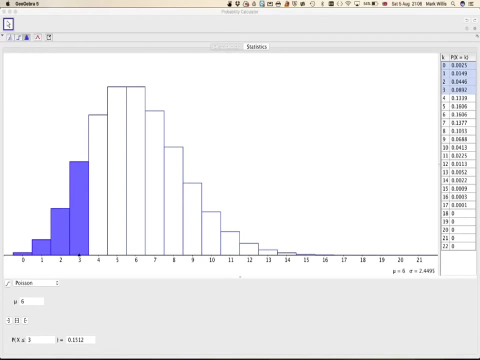 Therefore, Y will be plus or distributed, 6, minus, 6.. We want three or less. We want the probability that Y is less than or equal to 3.. So using the PDF. so we go to GeoAlgebra. I've already set this up. You should know how to do it by now. 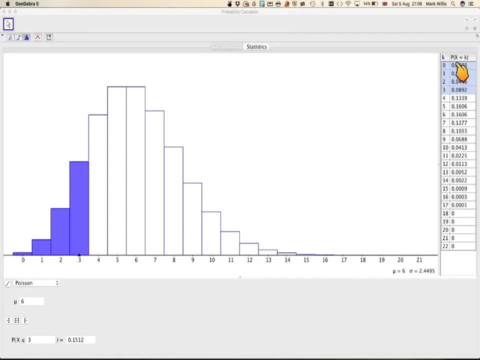 So we want less than 3.. So we would have to sum all these less than or equal to 3. So we have to sum all those probabilities up. Of course it's better to use The CDF, which is 0.1512.. 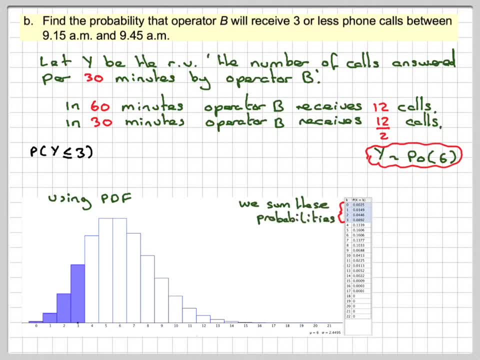 Screenshot of that. However, better to use the CDF and we get 0.1512.. So 0.1512.. And we'd round that off to three significant figures to get 0.15123. significant figures. Now we have to find the probability between them. 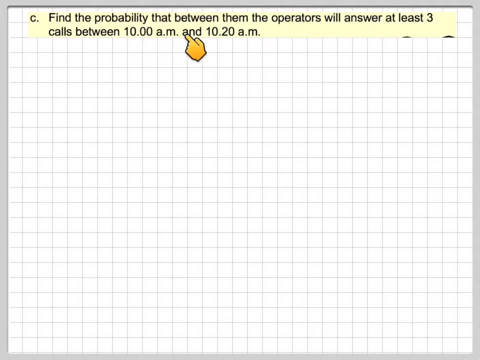 Operators will answer at least three calls between 10 am and 10.20 am, So let T be the random variable, the total number of calls answered by both operators, A and B, in 20 minutes. now, This is the time period. 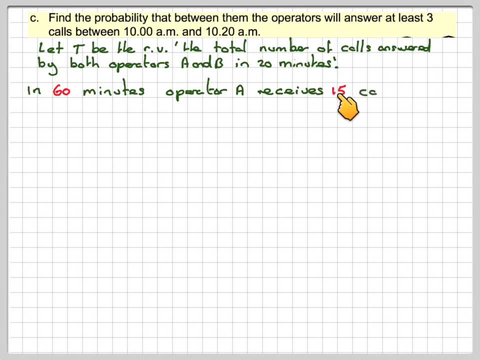 So in 60 minutes operator A receives 15 calls. according to the question, Therefore, in 20 minutes he receives 15 divided by 3 calls, which is 5.. And then for operator B: in 60 minutes operator B receives 12 calls. 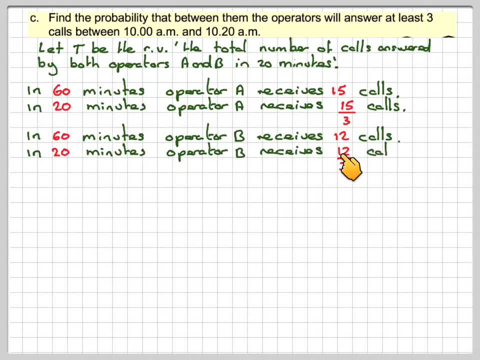 And then in 20 minutes, operator B receives 12 over 3 calls. So T will be Poisson, This is going to be 5, and this is going to be 4.. 5 plus 4., So in total they're going to receive 9 calls.